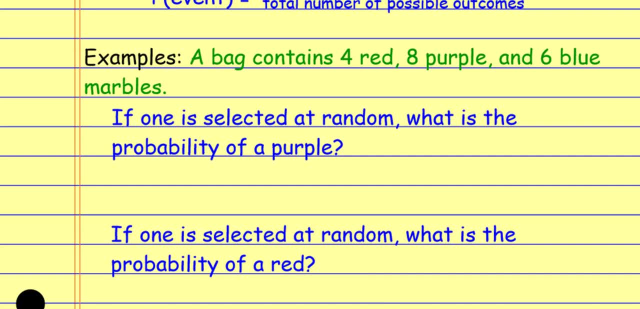 I could get a purple marble if I pull any one of those eight purple marbles, So it's eight out of the total number of options. Well, if the bag has four red, eight purple and six blue marbles, there's a total of 18 marbles in the bag And really I could get any one of those 18.. 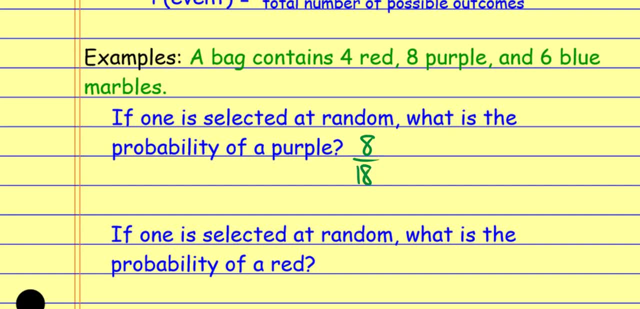 So, in terms of the total possible options, there's 18 total possible options, So the probability is eight out of 18.. And, of course, I have to get eight marbles in the bag. So I have to get eight marbles in the bag. 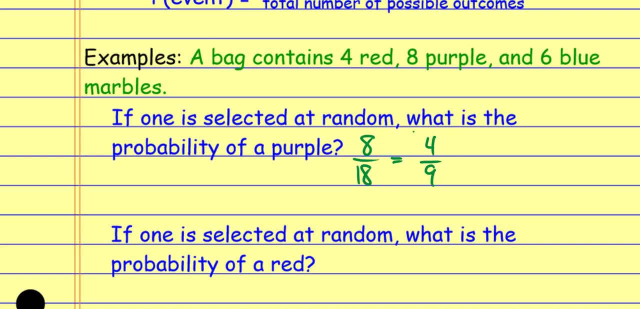 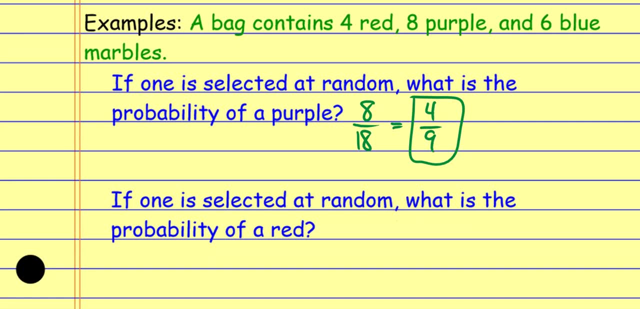 I have to reduce that fraction, So it's going to be four out of nine. Okay, Look at the next one. Same kind of setup. here. We're using that same bag. If one is selected random, what is the probability of a red marble this time? 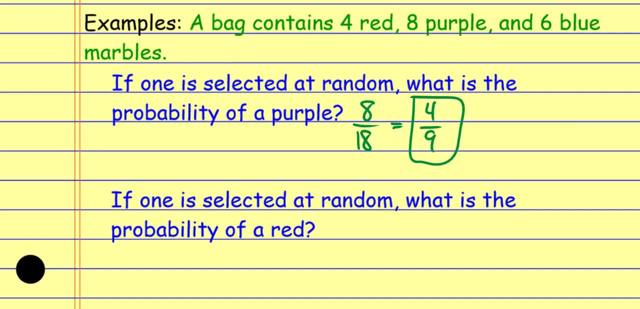 So the number of ways that I could get a red marble. there are four red marbles. I could get any one of those four. So there are four options for me to get a red marble And once again there are still a total of 18 marbles in the bag. So there's still a total of 18 options. 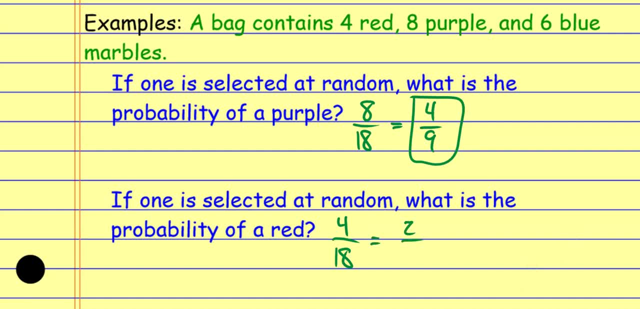 that I could potentially get, And once again, you have to reduce that. So that's two over nine. Okay, So that's just simple probability in a nutshell. Okay, It's what can give me what I'm asking for or what I want. over how many total options are there? 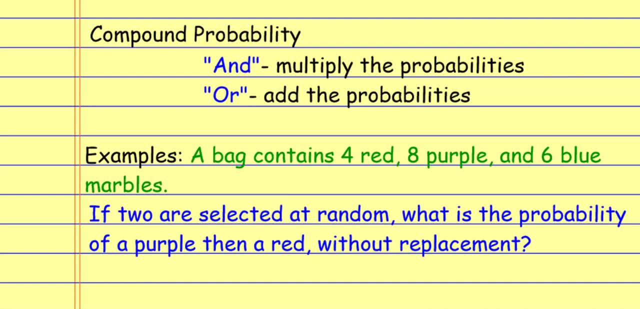 Then talk about compound probability. Compound probability is when we have the word and or the word or thrown in there, And when we have an and probability, we're going to multiply the probabilities, And when we have an or, we're going to add the probabilities. So, if I have kind, 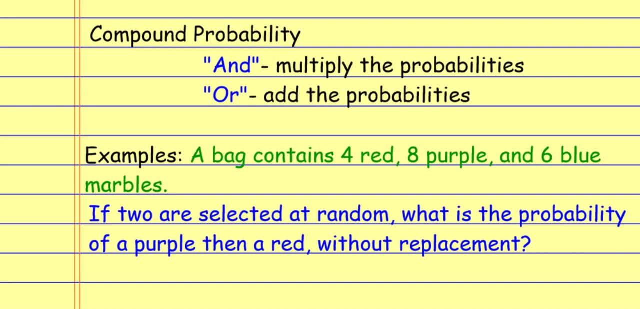 of two events. I'm going to have two events. I'm going to have two events. I'm going to have two events happening, two things that I want to have happen, And I say, what's the probability of this thing and this thing? Well, I would find the probability of each of those things and then 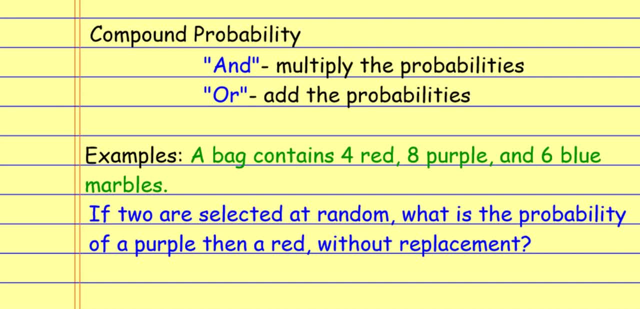 multiply them to get the probability of both of those things. Okay, So I look at the probability of each thing individually And if I want them to happen together, if there's an, and I multiply to get the probability of both things happening together. All right, An or probability same. 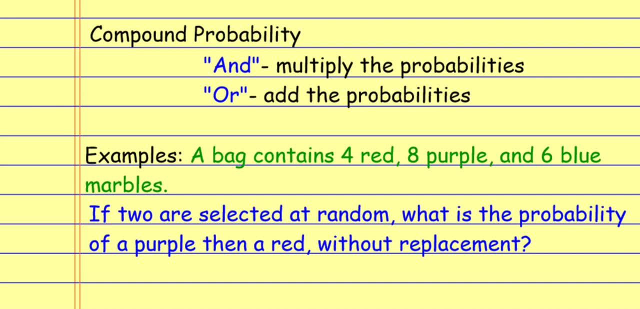 kind of thing: If I have two different things that could happen, I would say what's the probability of this thing or this thing? I would say what's the probability of this thing or this thing? I just look at those individual probabilities and say, hey, if I can get one or the other. 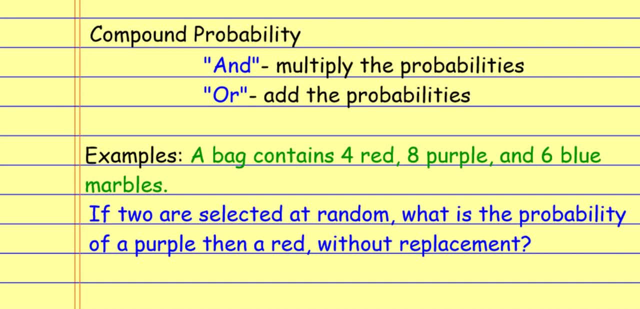 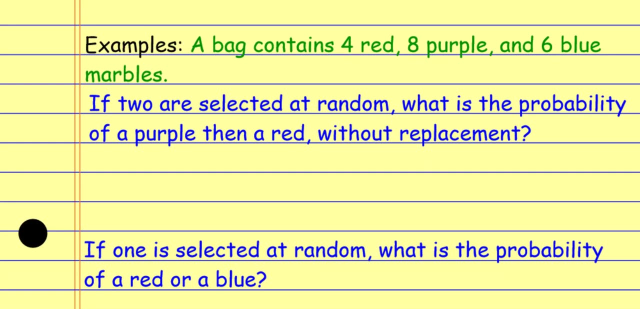 let's add these together to give me the probability of getting either one. Okay So, and is multiply because I want to get both, or is add because I want to get one or the other. Okay. For example, once again same kind of setup here I've got a bag that has four red, eight purple and six blue. 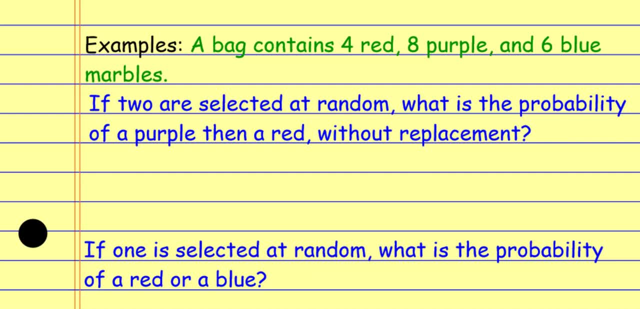 marbles. If two are selected at random this time, what is the probability of a purple marble, Then a red marble and without replacement? So a couple of things here. Notice, we don't actually see the word and, but the word then implies the word and. Okay, If I'm thinking about this as either an and. 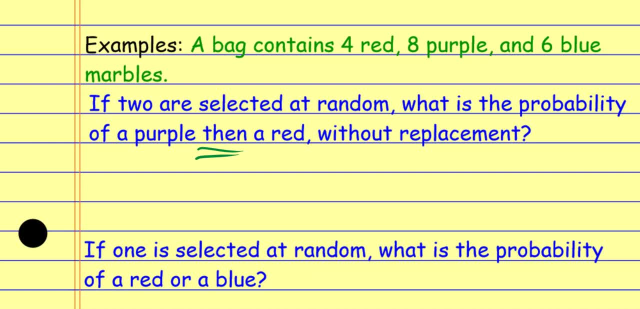 or an, or probability. it wouldn't be a purple or then a red. It would be a purple and and then a red. Okay, So the word and is implied, And then the other thing that I have to look out for here is this: with replace, sorry, without replacement, That just means, if I take the first marble out, 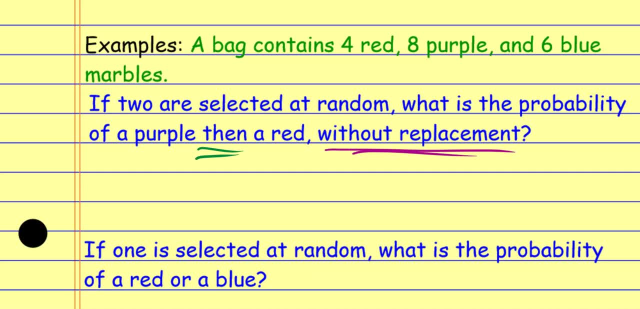 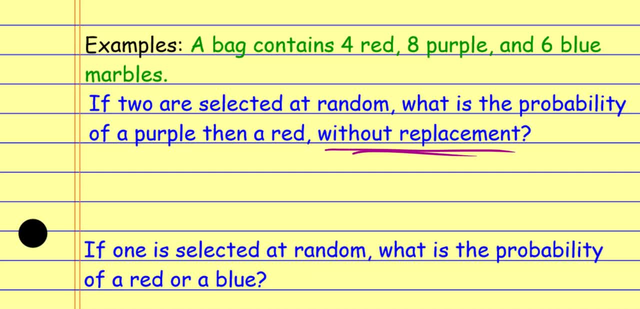 to kind of use my imagination a little bit. And so for this one I want a purple marble, then a red marble. So the purple marble. I'd already solved this once, but I'll do it again. So for the purple marble I would say, okay, that's eight out of 18.. There are eight purple marbles out of 18 total. 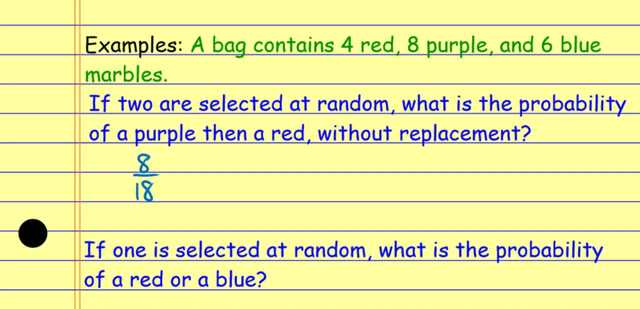 options. Okay, But now, before I move on to the probability of the red marble, I have to use my imagination. I have to pretend that this first thing has happened, that I actually pulled a purple marble out of this bag. And so if this is my bag, right here and I pull one of these, 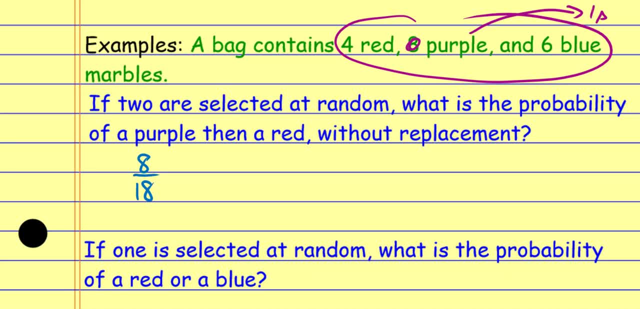 purple marbles out. what happens now is I only have seven purple marbles left in the bag because I pulled one of them out And then, when I look at the total, I only have a total of 17 marbles left in the bag. Okay, So there's two things that happen there. I have less purple marbles in. 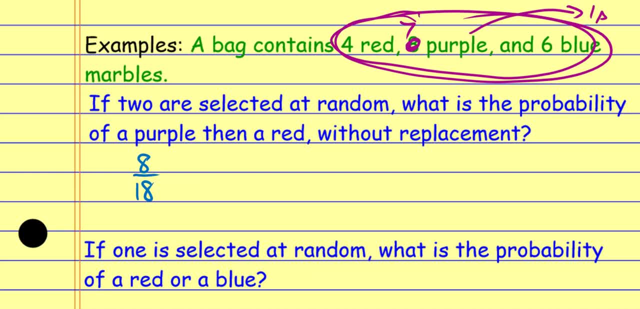 the bag and I have less total marbles in the bag. So now let's talk about the probability of a red marble. So if I look at the contents of the bag, there are still four red marbles in the bag, So four out of well. there's only eight, sorry- 17 total marbles left in the bag, So out of 17.. 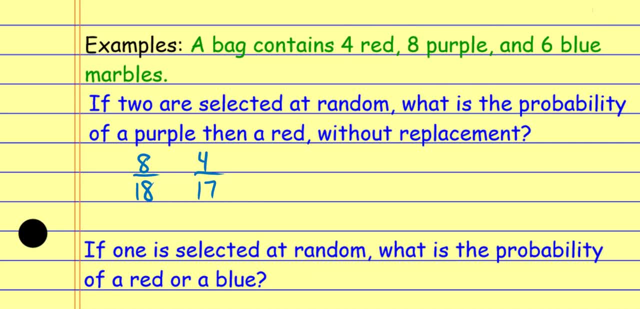 Okay, So you just have to kind of take these one at a time, use your imagination a little bit And if it helps to draw a picture, go for it. And now, because it was a purple and then a red, so and means I multiply the probabilities. I'm going to go ahead and simplify this a little. 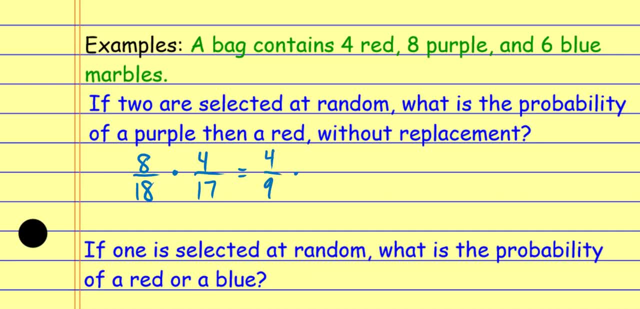 bit. first, That's going to be a four out of nine and then times the four out of 17.. And uh, you know this is a job for the calculator. If you need to do the nine times 17, here it's a one 53.. Okay, So the probability is 16 out of one 53.. 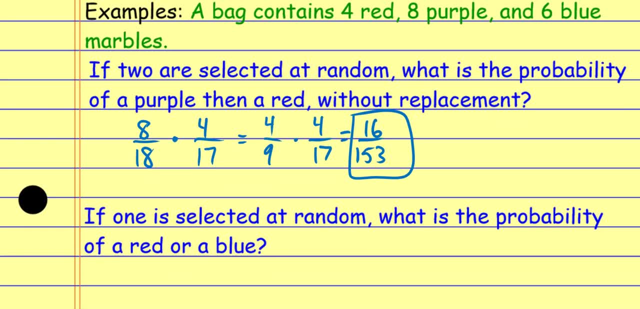 If I look at the next, one says one is selected random. What is the probability of a red or a blue marble? And so, once again, when I look at this one or means I'm just going to add these probabilities, And since I'm only pulling one marble, it's like I'm looking at two completely. 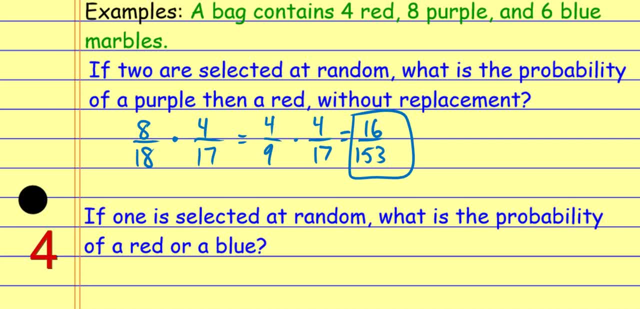 different cases. It's not like the previous one, where I'm actually doing this first thing And now I'm seeing what happens with the second thing. I'm kind of almost looking at hypothetical situations. Hypothetically, if I pulled a red, if I wanted a red marble. 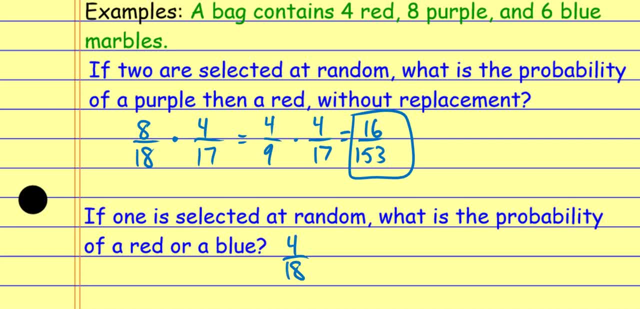 well, the probability would be four out of 18, but then separately, let's pretend that, pretend that didn't actually happen. Hypothetically, what's the probability? of a blue marble would be six out of 18.. Okay, Or means we're going to add these And one of the things that's different. 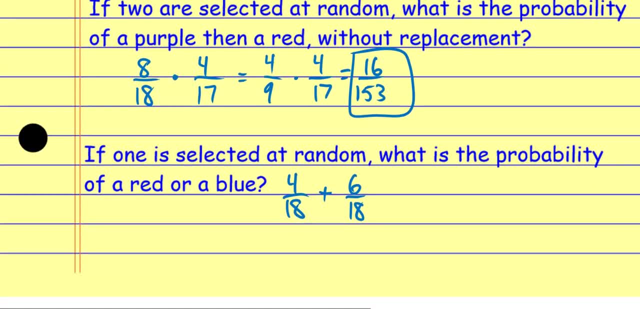 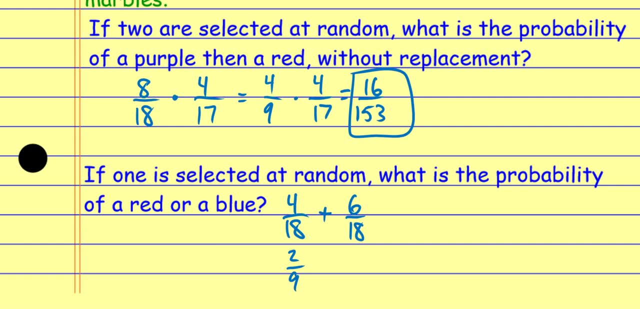 here. in the previous example I simplified before I multiplied. Here I don't want to simplify before I add. Watch what happens if I simplify each of these fractions. This is a two over nine. This one is a one out of three. Now to add these. well. 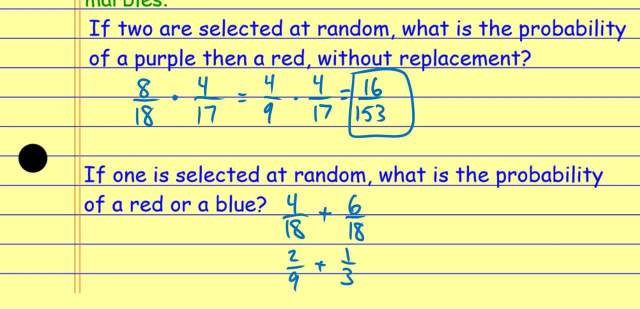 I can't add these the way there are. I have to get common denominators. Well, I already had common denominators before. I ruined it by simplifying. Right here I have common denominators, Let's add them the way they are. I add the numerators denominator stays the same. Now 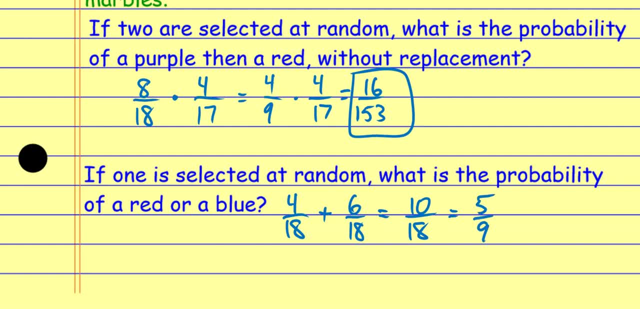 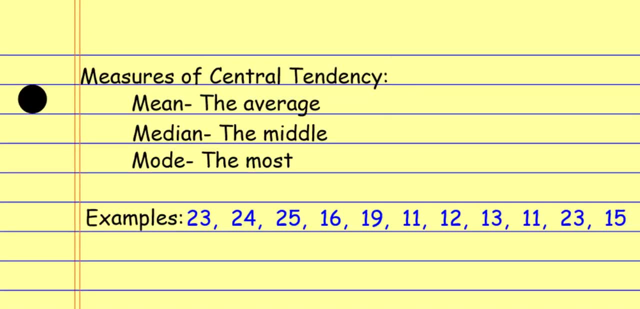 let's reduce this thing. Okay, Don't mess up your common denominators. Add them together in there And reduce. Okay, Statistical measurements. One of the big things here is measures of central tendency. Remember it's the mean, mean and the mode And the quick, easy way to remember these. 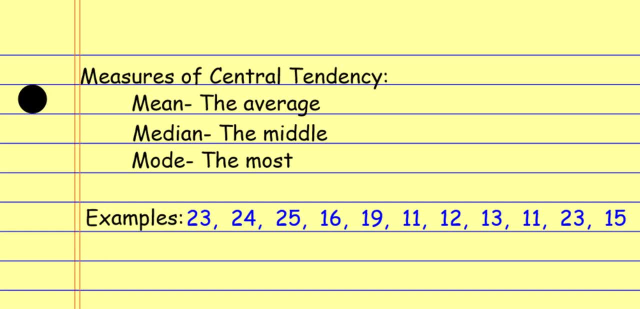 instead of going to the full definitions, is the mean? is just the average. When we average things out, it's always add them all up, divide by how many we have. That's the average. That's how we average our grades. That's how we find averages in anything. Okay, Add them up, divide by how many. 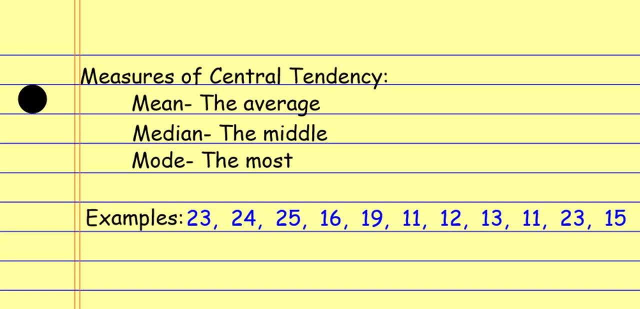 you have. So the mean is the average, The median is the middle. Remember, we line up the data values in order. We find the middle value And if there's a tie, we find the middle of those two middle values And the mode is the. 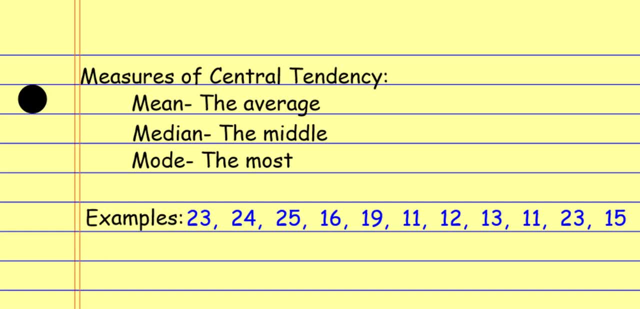 most. Okay, So it's the one that appears the most often. And remember, with the mode, if nothing is repeated, then there is no mode. But if two things are tied for the most because they are repeated, then I have more than one mode. Okay, So just keep that in mind. So mean median mode. 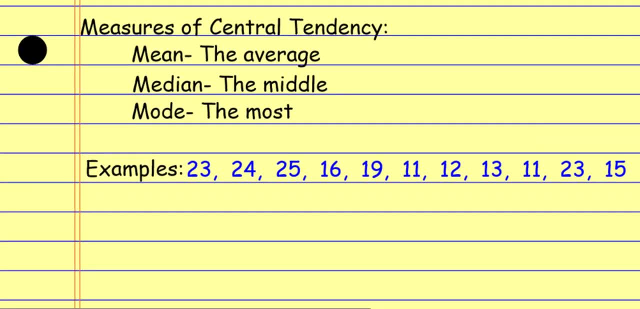 the average, the middle and the most. So I look at something like this guy. Once again, if I want to do the average of this thing, I just add them all up. So here I'm just going to add all these together and then divide by how many I have. 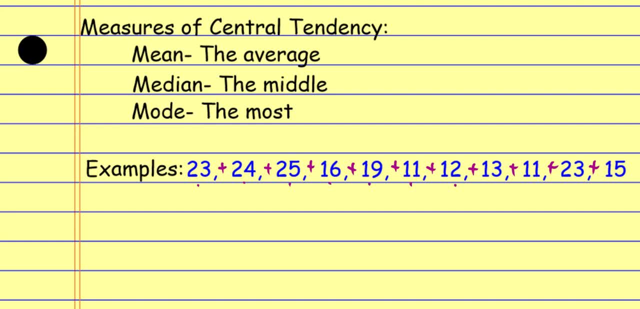 And it looks like I have 1,, 2,, 3,, 4,, 5,, 6,, 7,, 8,, 9,, 10,, 11 of these things. So I'm going to add them all up and divide by 11.. And so this is just a job for my calculator, So I'm going to go ahead. 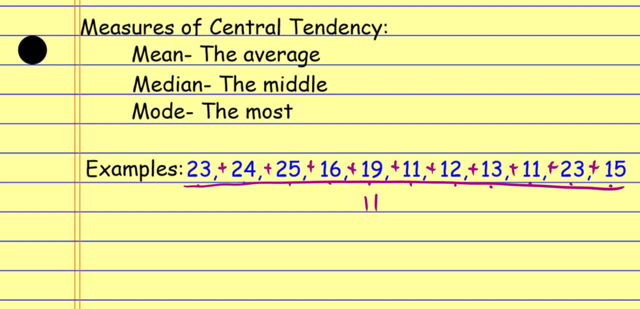 and plug this in. And when I plug this one all in, I get for the mean, and I'll denote it this way. so the mean, or I guess I could just call it the mean like this: okay, that's the symbol, that x with a bar over it, but I get a 17.45, and then 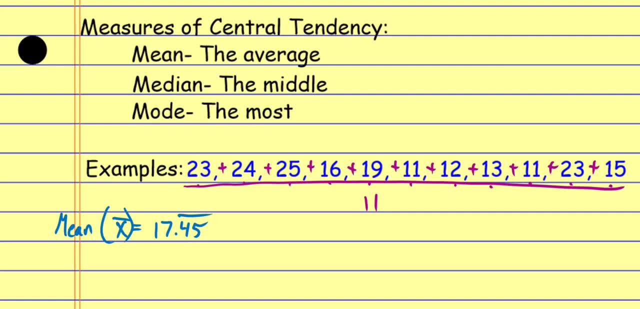 the 45 repeats kind of forever and you know, depending on the question, it might ask for the exact value. it might ask you to round this thing off, okay. so there's the mean. it's that 17.45 repeating now the median. the median to me is the worst one to have to do, especially when there's 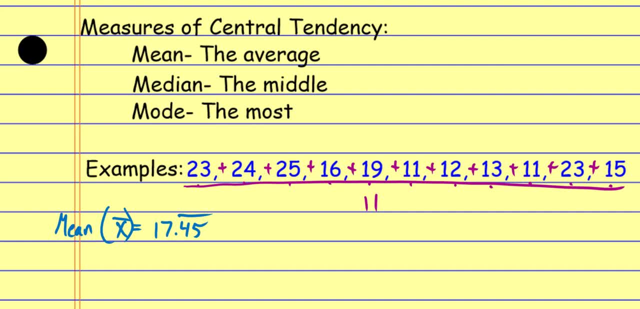 lots of data values, because the first thing I have to do is I have to reorganize this, so I have to write all of these in order. so let me reorganize this list. so I'm going to start with the smallest. 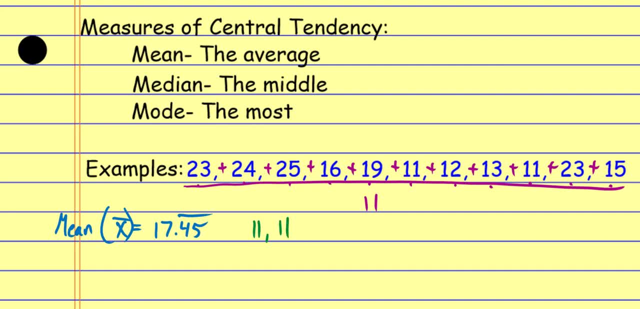 it looks like the smallest is 11,, looks like I have another 11,, so I'll just cross these off as I go. and then the 12,, the 13,, looks like 15 is next 16, 19,, and you know, we always kind of run. 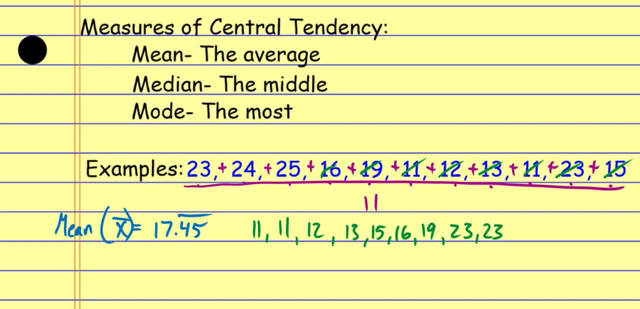 the risk of- oh what if we miss one? There's two 23s, And that happens to me all the time, Like I'll miss one and then have to kind of reorganize my list just a little bit to squeeze it in there. And one of the things I like to do is 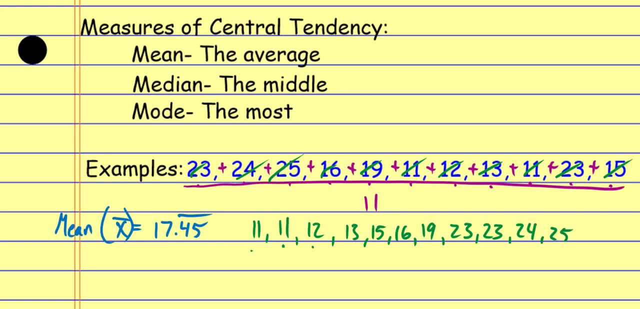 I always like to just double check. count the values you have: 1,, 2,, 3,, 4,, 5,, 6,, 7,, 8,, 9,, 10,, 11.. Okay, And I know I'm supposed to have 11 values. It's not a foolproof way of making sure. 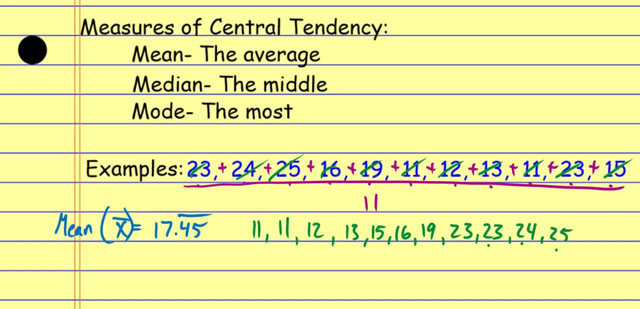 that nothing has gone wrong here, But it's a nice little quick check, Okay, And so now I count to the middle. All right, I have 11 data values. So if I start kind of marking these off on each end, here's the two ends. And now, counting in from each end, mark the third one on each end. 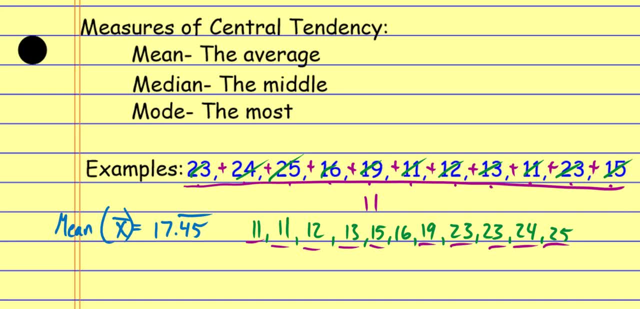 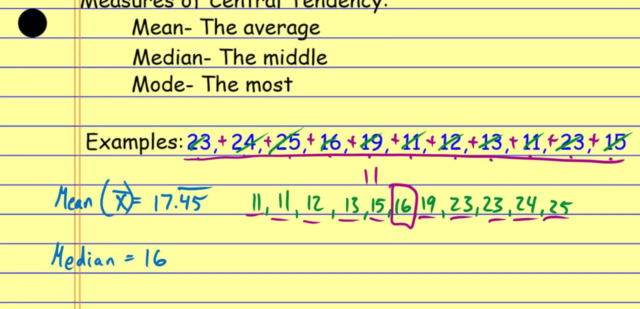 the fourth one on each end, the fifth one on each end, And what I'm left with is this guy in the middle, So the 16.. Okay, So that's my median, Uh, the mode. I could go back to the original list, but the mode is actually easier to identify. 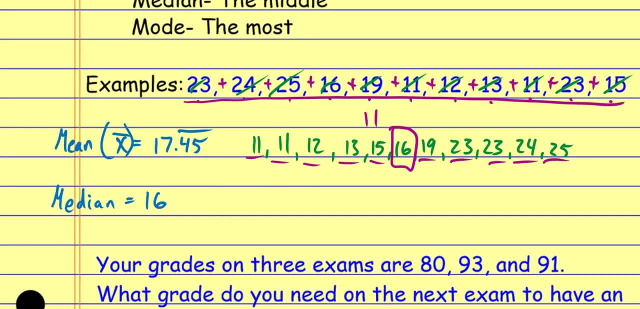 when we have this thing organized. So, just like what I do with the median, if I look at the organized list here, it looks like I have two values that are repeated and it's these guys. So, right here, the 11s, there's two of those in the 23,. there's two of 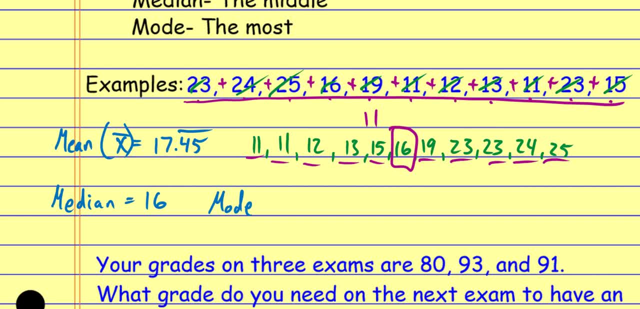 those, And since neither one of those kind of wins out, they're tied. I have two modes this time. The mode is 11, but it's also 23.. So there are two modes this time. Okay, But that's it. Mean median mode. 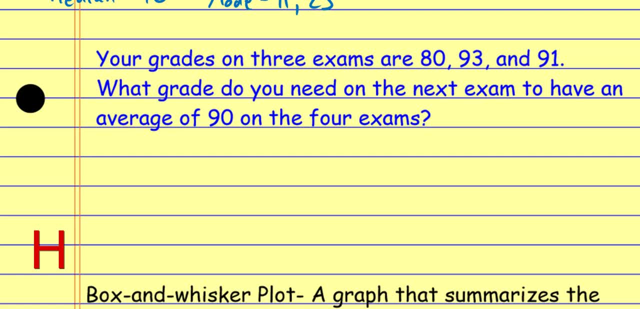 Something like this guy. it says your grades on the on three exams are 80,, 93, and 91. What grade do you need on the next exam to have an average of 90 on all four exams? And so really what I have here is I have three exams listed, but I'm talking about 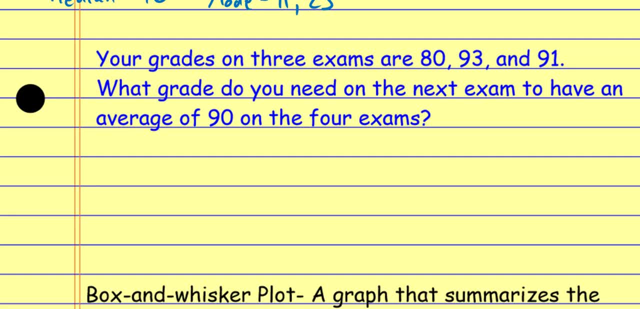 four exams total, And so if I, if I look at it this way, if I write down my exams, it's 80,, the 93 and the 91, and then some unknown exam, I'll call it X. Okay, Those are the four exams. I want the average of. 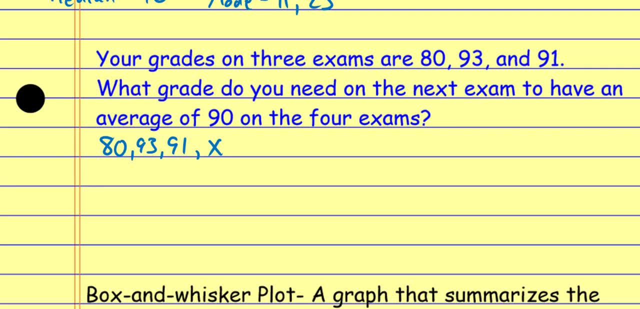 And so if I want the average of those four exams, well, the average of those is well, add them together. So add those four together and divide by how many I have, which, I've already stated a couple of times, is four exams. Yes, I don't know what one of them is going to be yet. 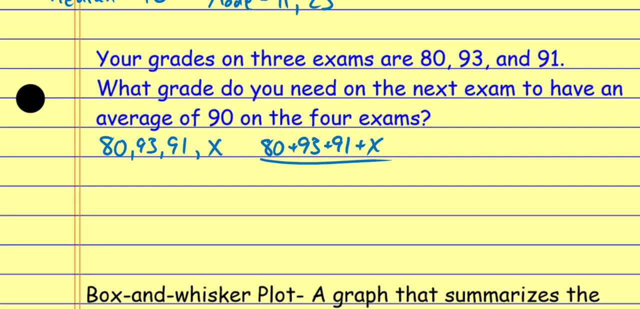 but that's the fourth exam I want to include in this average. Okay, So I have to include all of them, even the unknown one, And I have to divide by the average. So I have to include all of them, divide by four, because I'm looking for the average of four exams, even though I don't know. 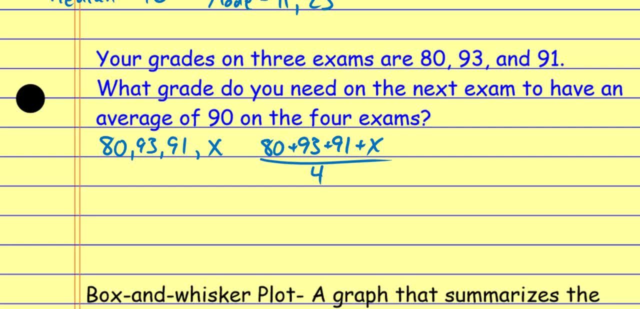 what the last one is yet Okay. And so this is the equation for the average right here is: adding them together, divide by how many I have. I want that average to equal a certain percent, a certain average, And the average that I want here is a 90. So I want that to equal a 90%. 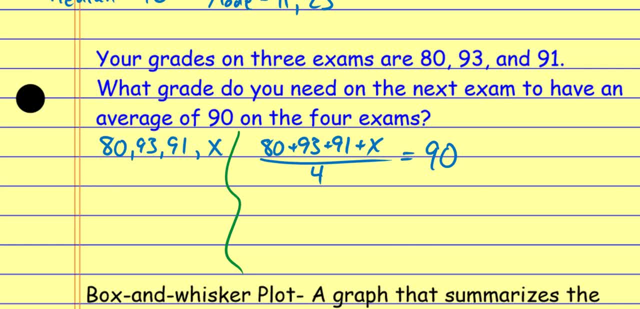 Now I'm going to solve this thing, Okay, And you could choose to solve this by cross multiplying. put that over one and cross multiply, or you can just multiply each side of the equation by four. Either way, you kind of get the same thing here. Let me combine these like: 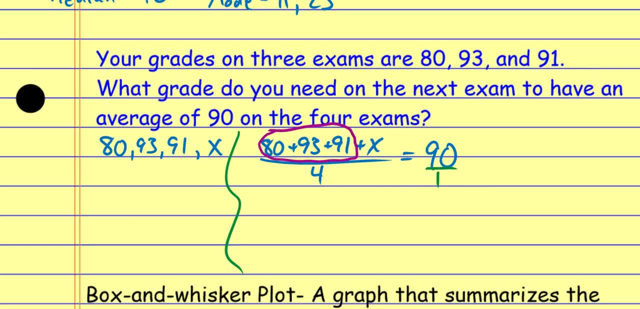 terms up here. So if I add those guys together it gives me a 264.. And if I'm cross multiplying here, it'd be that 264 plus X times one, which is just 264 plus X, And then the 90 times the four. 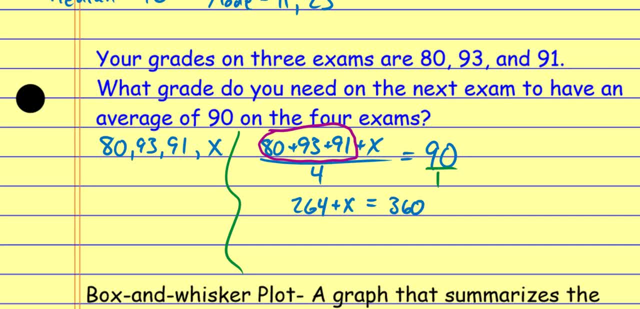 here And now I just solve what's left. I solve what's left over by subtracting the 264 from each side, And so it looks like the value I need on the last test is a 96%, which makes sense when you think. 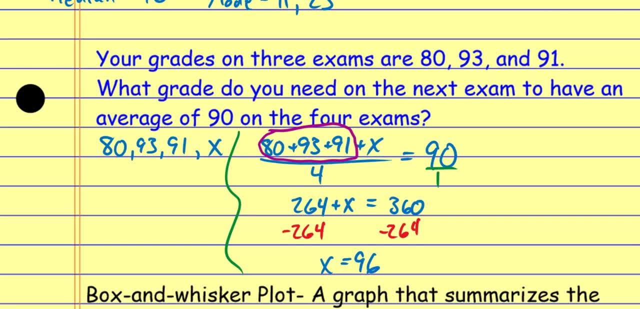 about it. I want to get a 90,, but that 80 is pretty low compared to the 93 and the 91.. All right, And so if I want an 80,, that- or sorry, a 90% average, that 80 is really going to be. 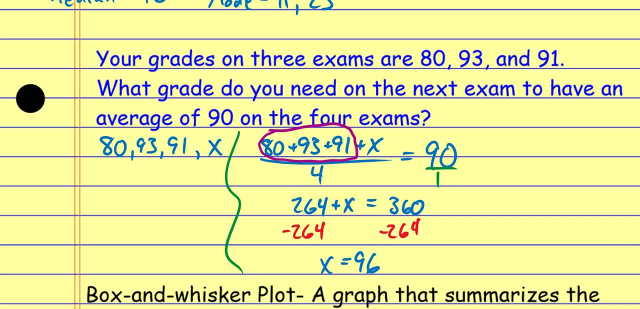 dragging things down, I'm going to need a pretty impressive score on this one in order to get a 90.. Okay, So the average we need is a 96% Okay, And if I get that, then I should have an average 90.. 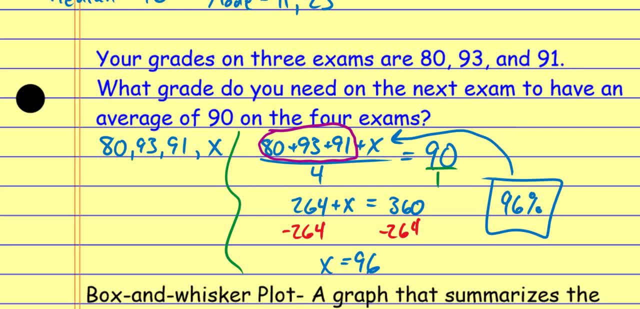 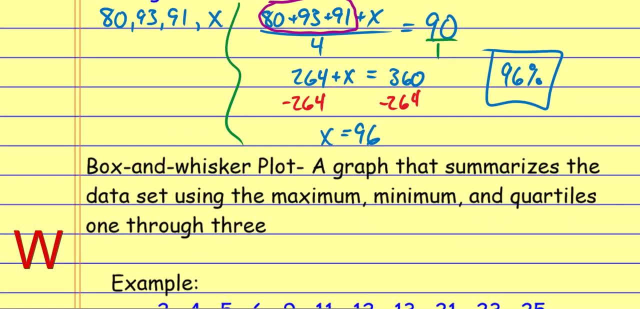 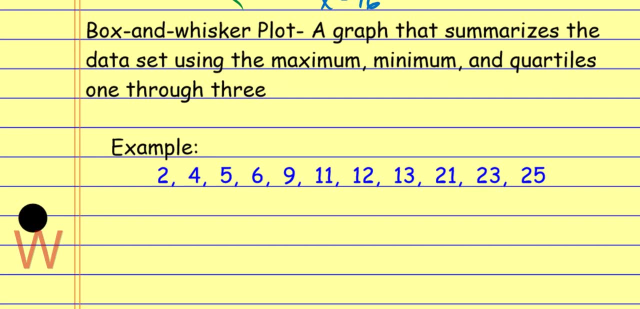 And this is easy enough to check. You can easily plug this back in and actually find the average of the four exams to make sure it equals 90.. Okay, This guy, a box and whisker plot. This is one of those things that you know it may. it forces us to find a lot of different values And 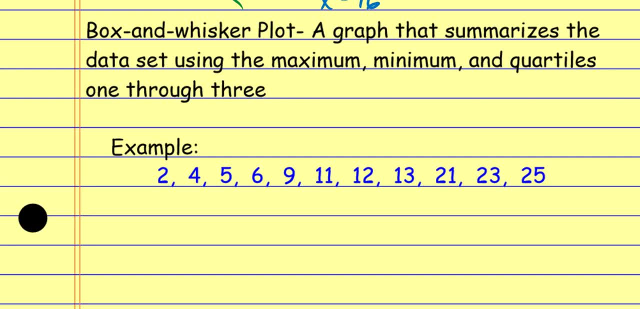 that's what's nice about this. It's not just a box and whisker plot. It's a box and whisker plot, But really it's kind of showing us a dispersion when we're looking at this thing. It's showing us how spread out the data is and where it might be spread out more than other places. Okay, 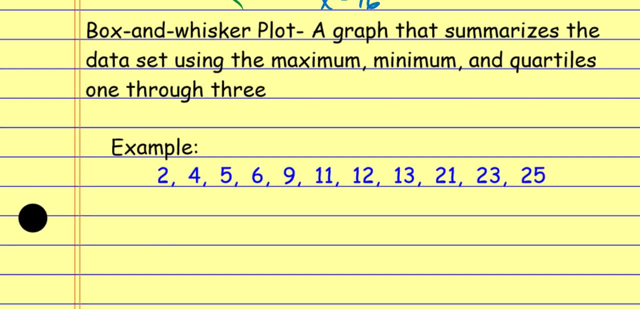 So here I'm going to create a box and whisker plot. Notice that the values are already in order for me, which is nice, And so what I do is I start identifying the quartiles. The quartiles, basically. I'm going to split this into four equal pieces, and it starts with the median. 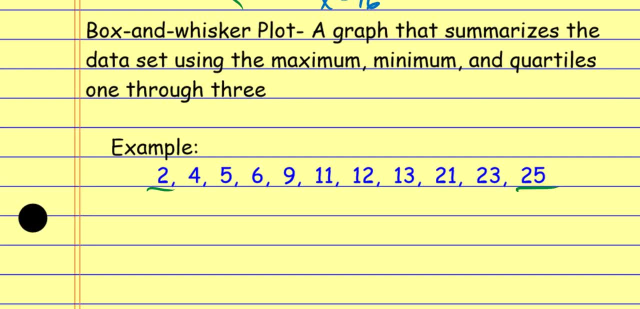 So I'm going to find the median. So I cross off from each end and notice I just underlined from each end, two on each end, three on each end, four on each end, five on each end. So the one in the middle, that's my median And really that's like my second quartile. So if you 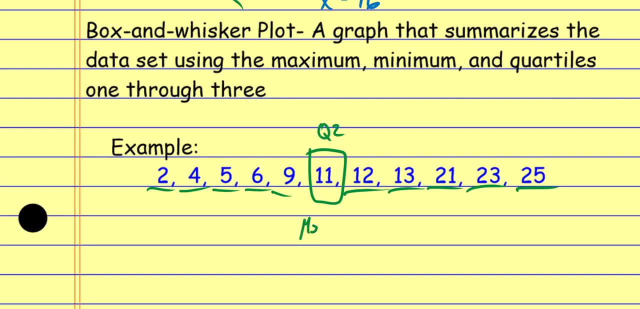 want to call this like the second quartile. well, that's the median. Okay, So that's 11.. But now I do the same thing, looking at each half of the data as its kind of own separate thing. I look at this half of the data and I say, hey, let's find the median. Then I look at this half. 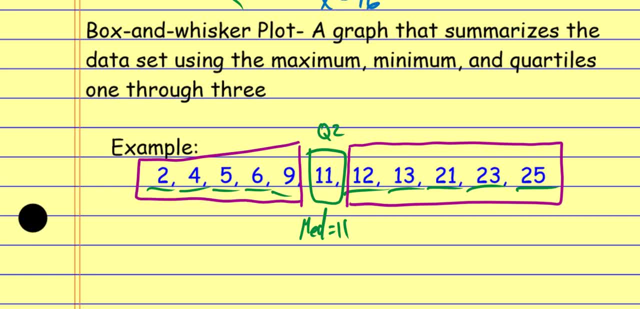 of the data again separately and find the median, And then I look at this half of the data again and those will give me the quartiles. So over here, as I kind of cross off from each end, one on each end, two on each end. the one in the middle is this guy, It's the five. 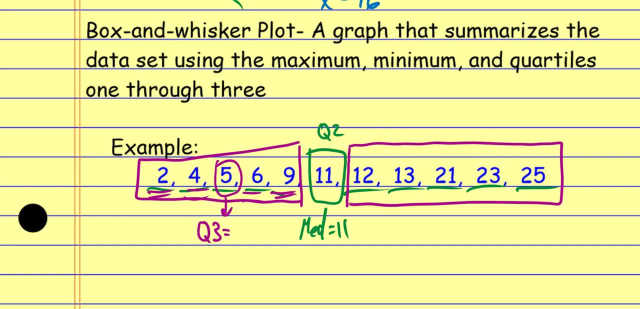 So that's the third quartile. Same thing on the other end. I cross one off on each end, two off on each end. The one in the middle is this guy. So that's the sorry. I've labeled this as the third. That's the first quartile. Got to pay attention to where I'm writing Over. here is the. 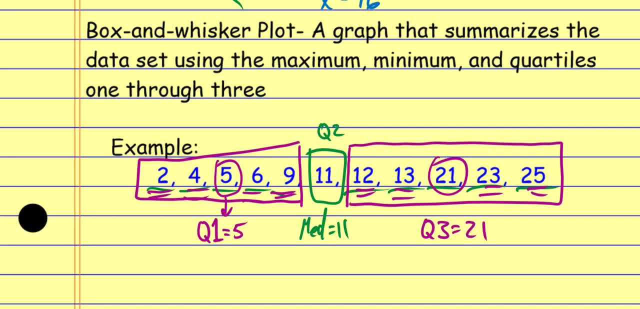 third quartile, 21.. And notice, these count up. You know we start here. If I kind of look at the progression here, the value on the end, that's the minimum, That's the two, That's the lowest value Over here. 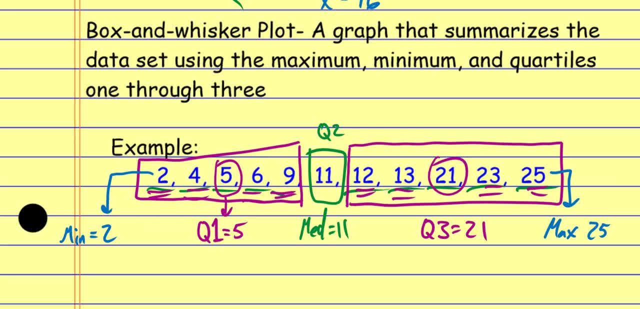 the value on the end. that's the maximum. Well, these should count up. Okay. The smallest value is two. Halfway through, the first half is five. Halfway across, all of the data is 11.. Three quarters of the way across the data is 21. And the whole way across the data is 25.. So it kind. 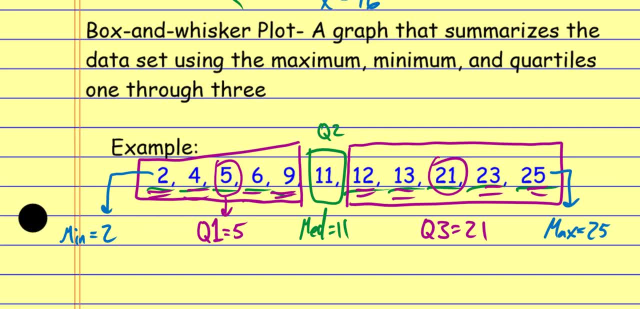 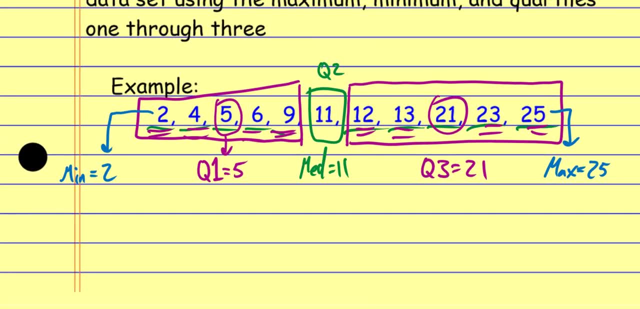 of marks, these increments Of where we collect a certain number of data values. Okay, And so now looking at a box and whisker plot. if I actually draw the box and whisker plot, it starts by drawing a number line. So we start. 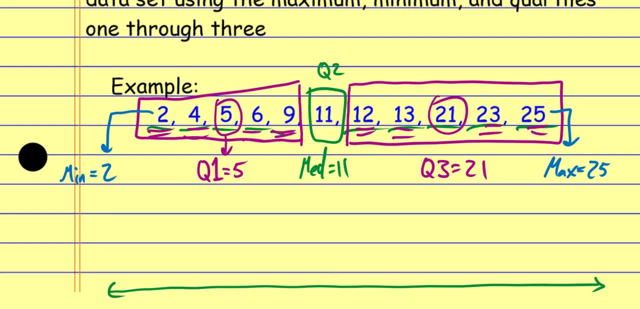 with a number line And it looks like I go from about two to 25.. Oh, it looks like it came up a little short. Let me just extend this guy just a little bit. There we go, And now I can go by one. So here I'll say: 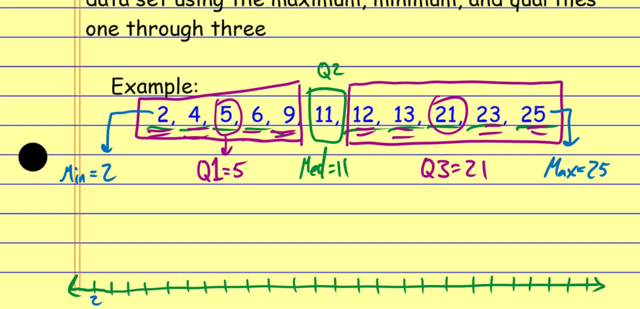 something like you know. this is the two down here, And now I'll label this by ones. Let's see 3, 4,, 5,, 6,, 7,, 8,, 9,, 10,, 11,, 12,, 13,, 14,, 15,, 16,, 17,, 18,, 19,, 20,, 21,, 22,, 23,, 24,, 25.. Okay, And I kind of 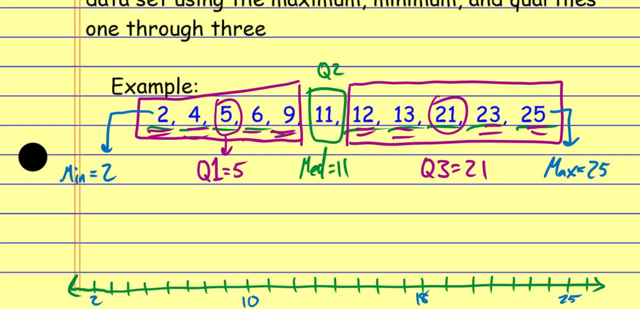 arbitrarily labeled some of those. I just threw some of the measurements down. I could label every one, But I just need to get a sense for where each of these values is going to be Okay. And so now, drawing my box and whisker plot, I plot this guy and this guy, the maximum and minimum, as kind. 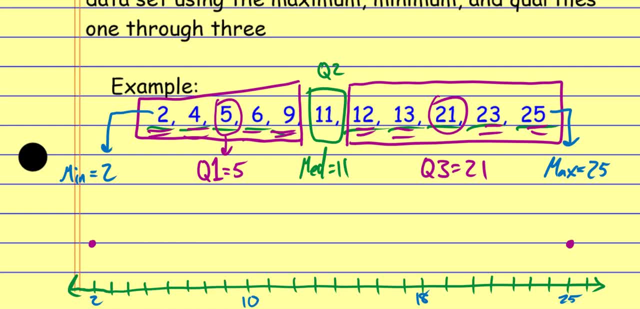 of points. I plot the first quartile as a line, which is right here. I plot the median as a line, which is right here. I plot the median as a line, which is right. here I plot the median as a line.